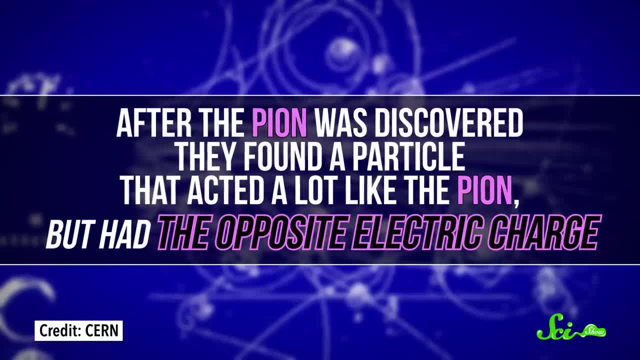 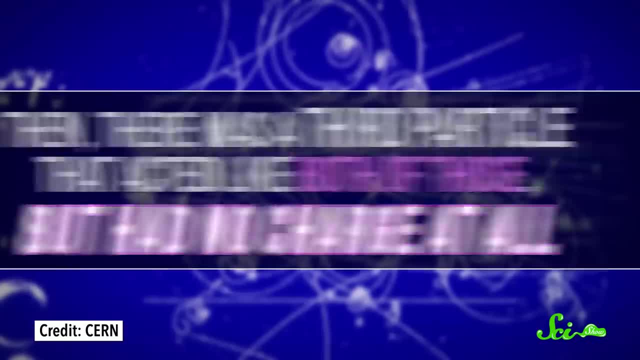 For example, after the pion was discovered, they found that the new particles were more like neutrons than neutrons. They found a particle that acted a lot like the pion but had the opposite electric charge. Then there was a third particle that acted like both of those but had no charge at all. 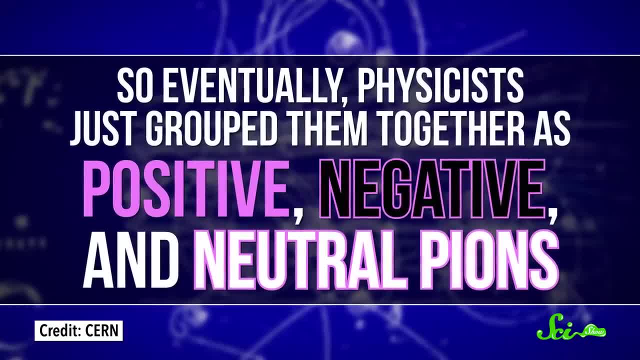 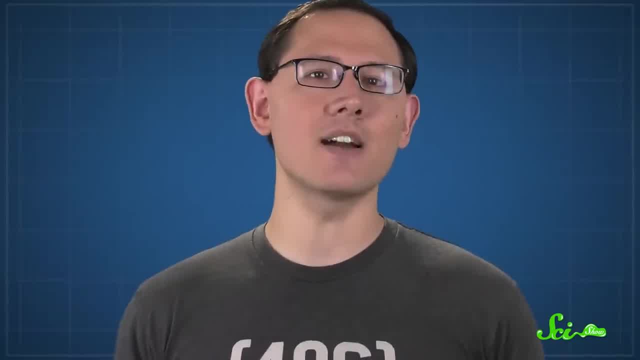 So eventually, physicists just grouped them together as positive, negative and neutral pions. Meanwhile, some particles like the kaon took strange-looking paths through particle detectors. So scientists said that the kaon had — and I'm not making this up — a quality called 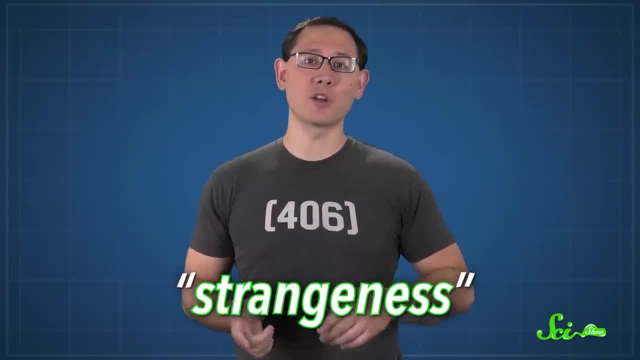 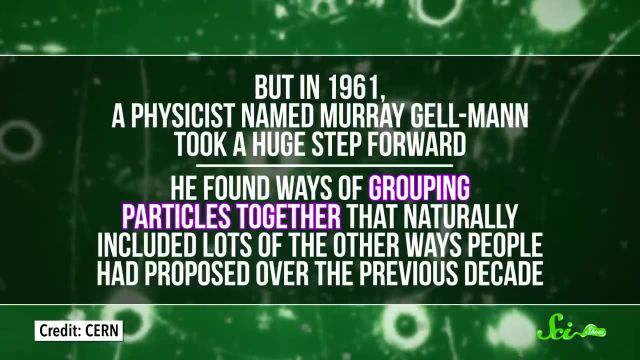 strangeness, And they grouped together particles with strangeness and particles without it. There were lots of other groupings floating around too, with different people thinking. different ones were more or less important, But in 1961, a physicist named Murray Gell-Mann took a huge step forward. 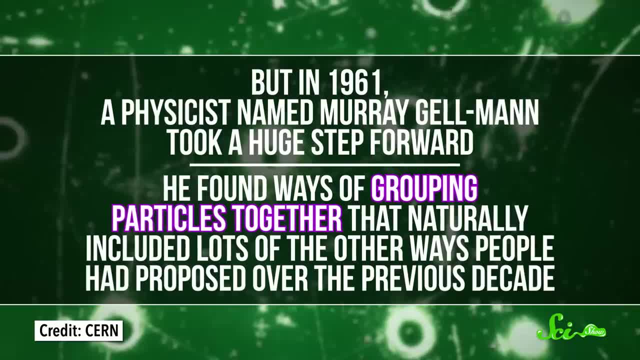 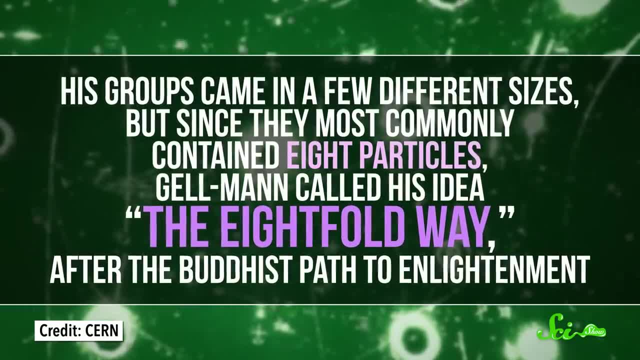 He found ways of grouping particles together that naturally included lots of the other ways people had proposed over the previous decade. His groups came in a few different sizes, but since they most commonly contained eight particles, Gell-Mann called his idea the Eightfold Way after the Buddhist path to enlightenment. 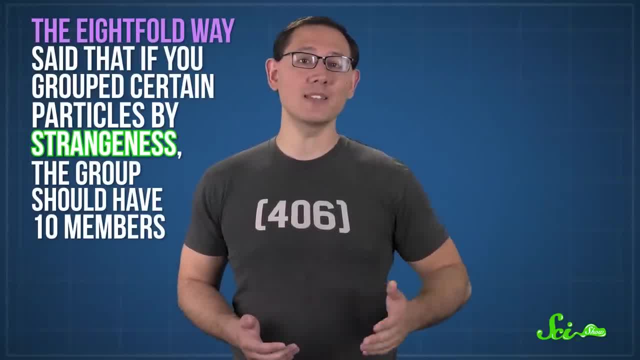 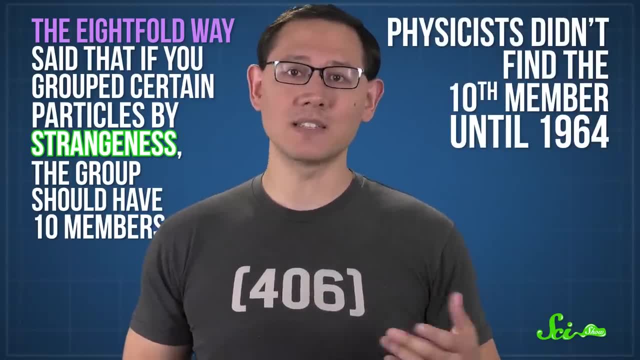 Some of his groups were incomplete, though. For example, the Eightfold Way said that if you grouped certain particles, by strangeness, the group should have ten members, But physicists didn't find the tenth member until 1964, a few years after Gell-Mann predicted. 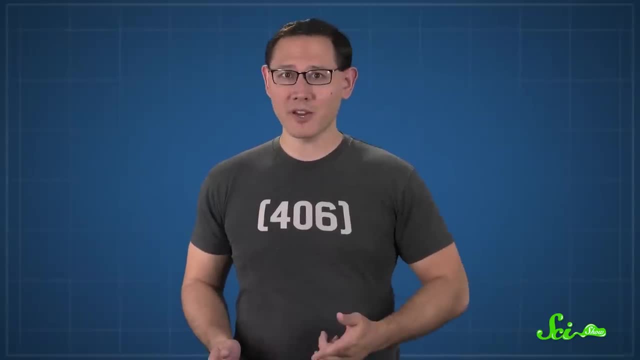 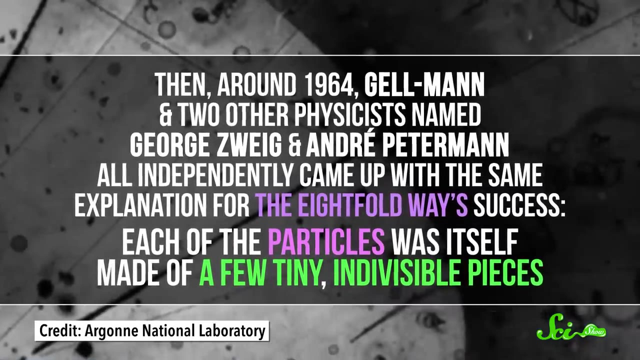 it Still. that was a good sign. Once they found that omega-minus baryon, as it's now known, everyone knew Gell-Mann was on the right track. Then, around 1964, Gell-Mann and two other physicists named George Zweig and Andre Petermann 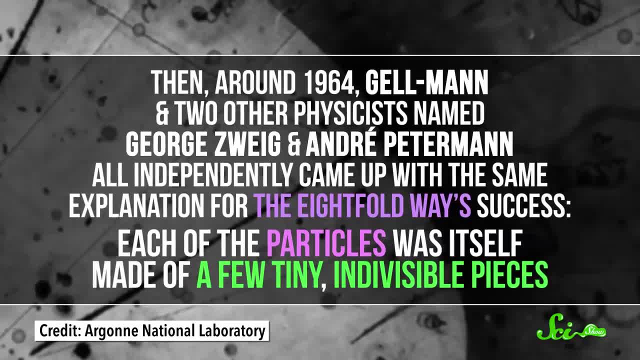 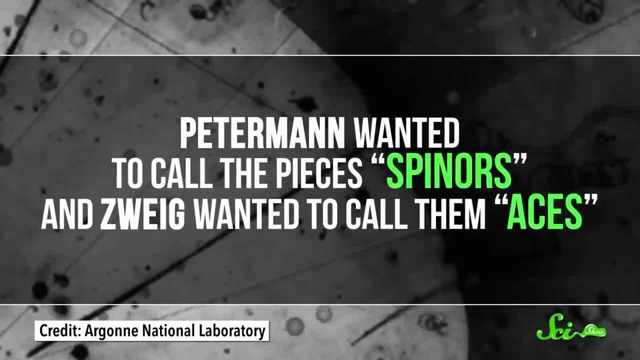 all independently came up with the same explanation for the Eightfold Way's success. Each of the particles was itself made of a few tiny, indivisible pieces. Petermann wanted to call the pieces spinners And Zweig wanted to call them aces. 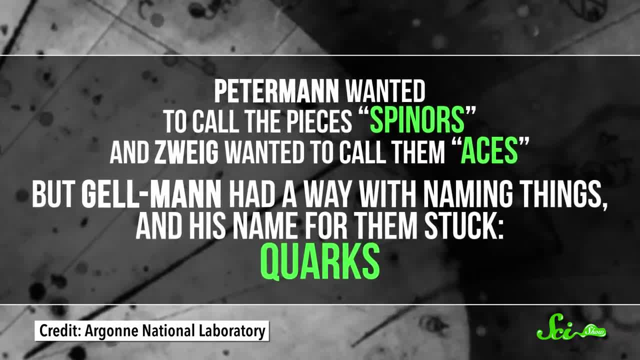 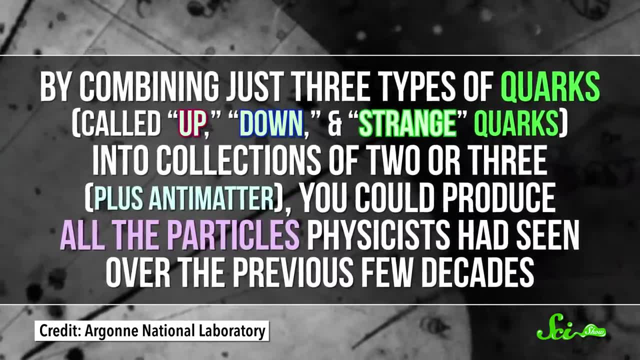 But Gell-Mann had a way with naming things, and his name for them stuck — quarks. By combining just three types of quarks, called up down and strange quarks, into collections of two or three, you could produce all the particles physicists had seen over the previous. 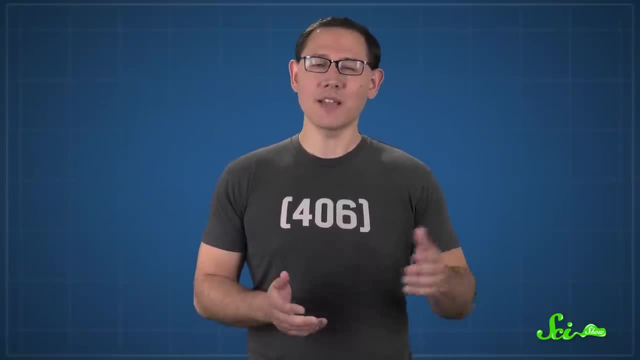 few decades, Except for things in the same family as electrons, But those have their own models, and there were only a couple of those at the time anyway. Admittedly, though, the quark model did have some weird features. It's said that, unlike every particle ever observed, quarks didn't have an electric charge, but they had a magnetic field. 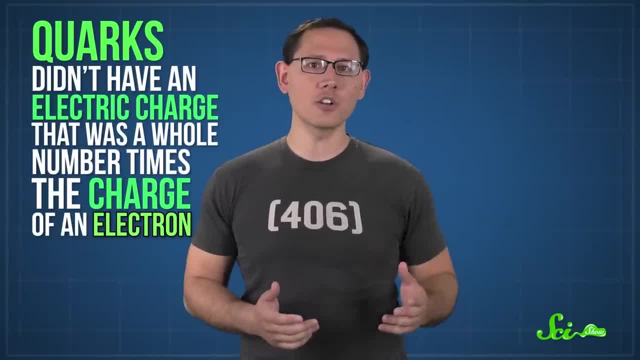 It's said that, unlike every particle ever observed, quarks didn't have an electric charge, but they had a magnetic field. It's said that, unlike every particle ever observed, quarks didn't have an electric charge, but they had a magnetic field. 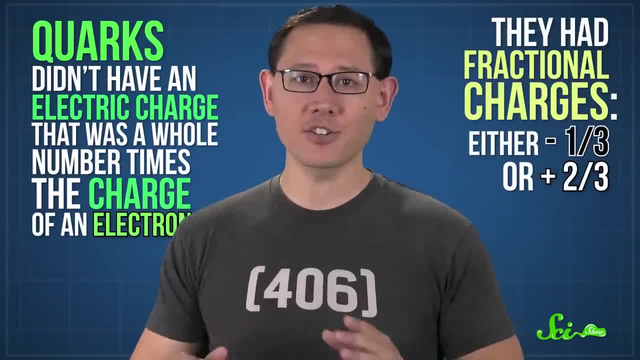 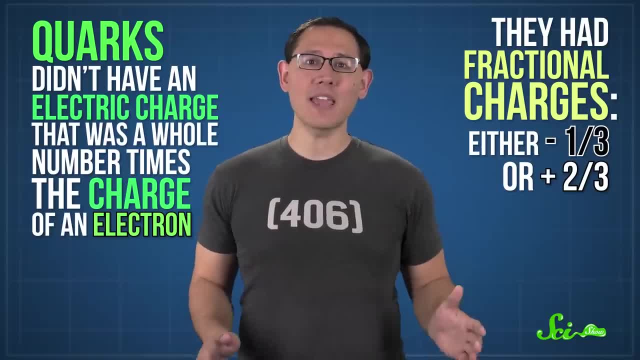 That was a whole number times the charge of an electron. Instead they had fractional charges — either negative one-third or positive two-thirds, And that struck everyone as very weird. It was unlike every particle they'd ever seen. But there was a reason. they'd never seen fractional charges. 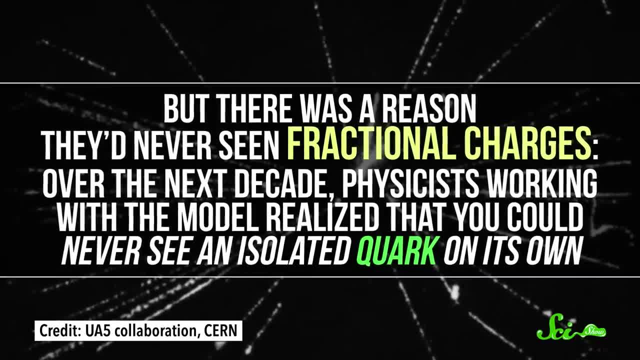 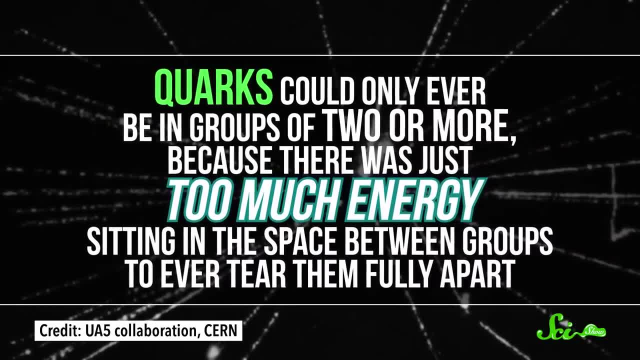 Over the next decade. physicists working with the model realized that you could never see an isolated quark on its own. Quarks could only ever be in groups of two or more, because there was just too much energy sitting in the space between groups. 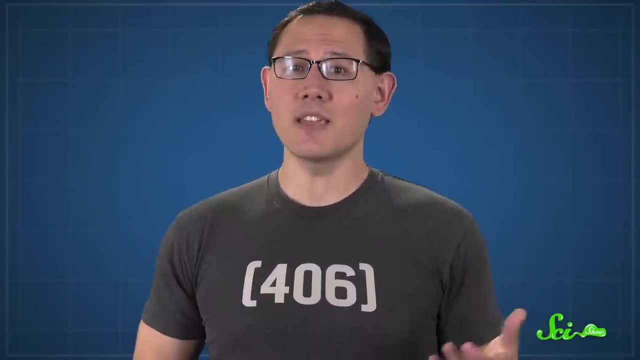 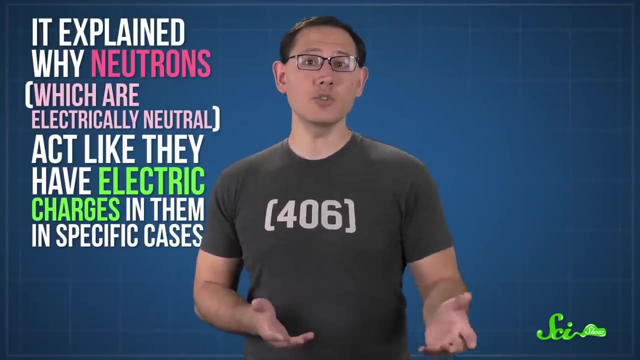 ever tear them fully apart Again. it's very weird, But just like the Eightfold Way, the quark model caught on because it worked. It was a simple explanation for complex mysteries. It explained why neutrons, which are, like the name says, electrically neutral, act like. 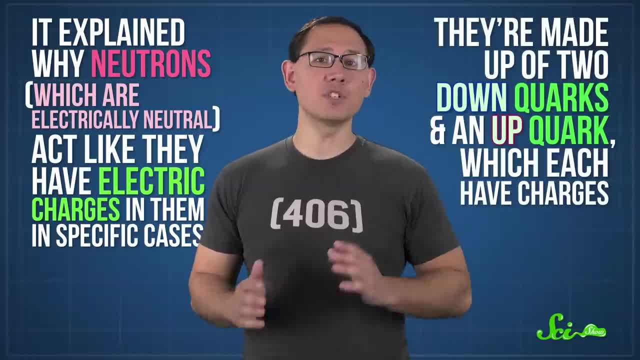 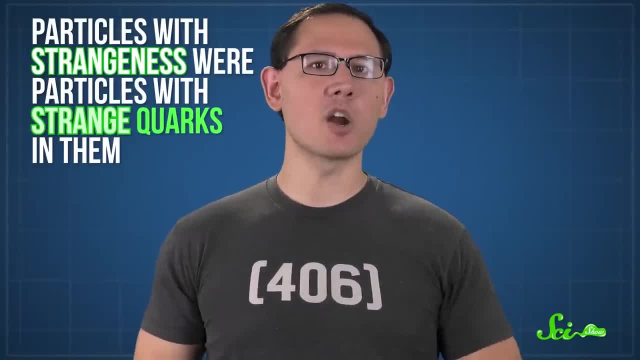 they have electric charges in them. in specific cases, They're made up of two down quarks and an up quark, which each have charges, And it naturally explains strangeness too. Particles with strangeness were particles with strange quarks in them. 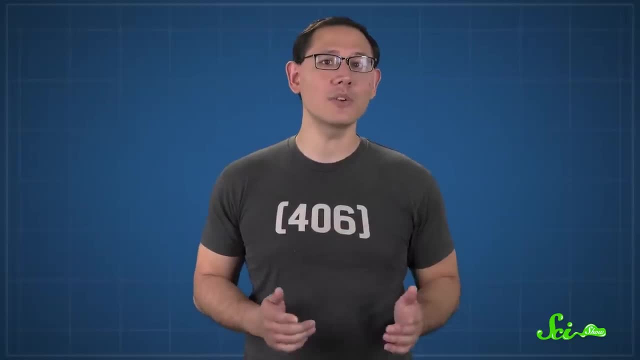 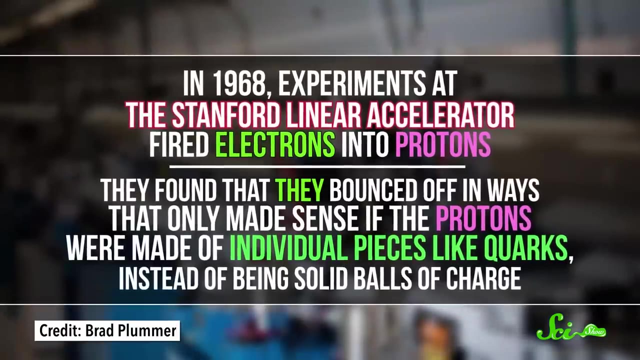 The real kickers came in 1968 and 1974, when two different experiments showed conclusive evidence that the quark model was right. In 1968, experiments at the Stanford Linear Accelerator fired electrons into protons. They found that they bounced off in ways that only made sense if the protons were made of. 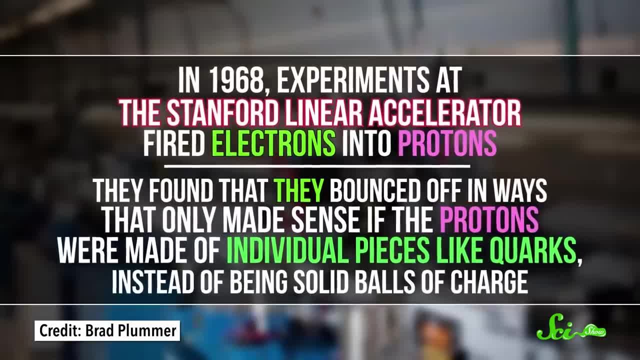 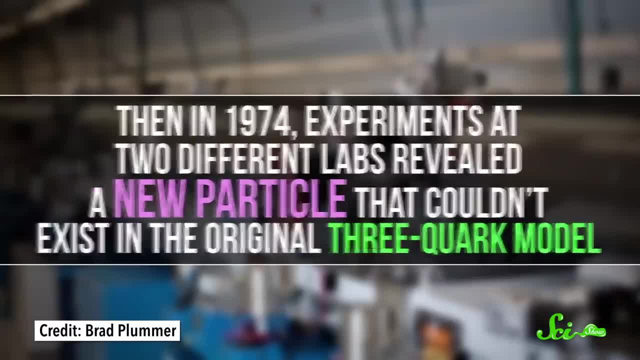 individual pieces like quarks, instead of being solid balls of charge. Then, in 1974, experiments at two different labs revealed a new particle that couldn't exist in the original three-quark model, Which would have been a disaster if physicists hadn't already 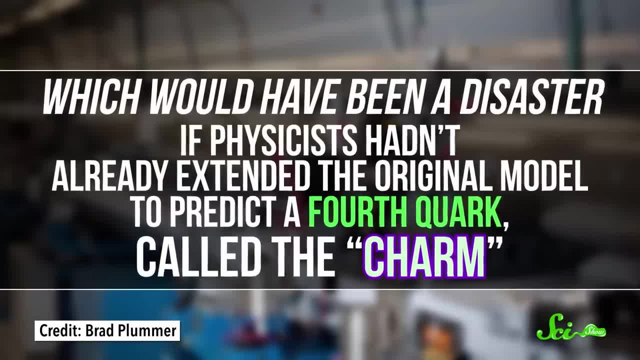 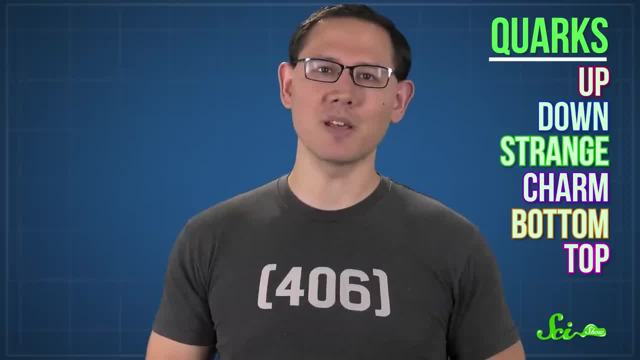 extended the quark model. They extended the original model to predict a fourth quark called the charm. Today we know of only two more quarks, the bottom quark and the top quark, which were originally called truth and beauty. but apparently that was just too much. 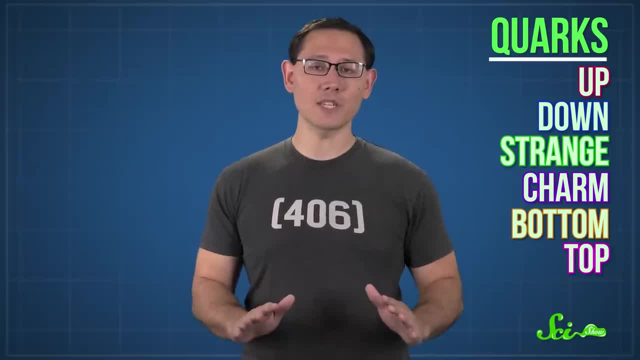 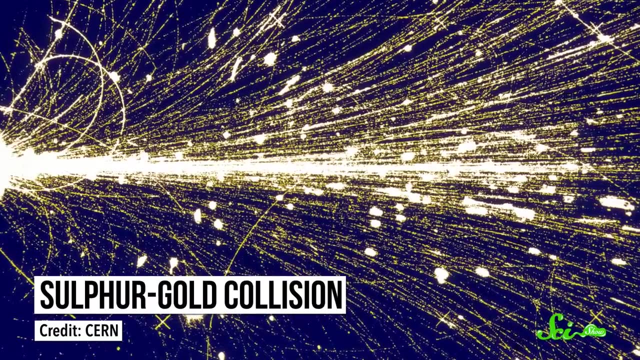 And there are good reasons to think that that's it. Our universe has six total types of quarks and no more. With just those quarks plus the forces between them and a couple other particles that are cousins of the electron, we can figure out a ton. 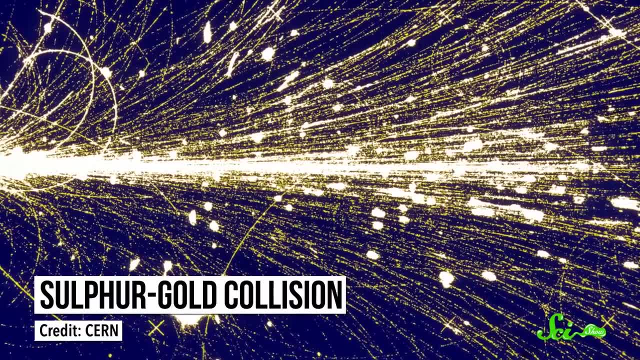 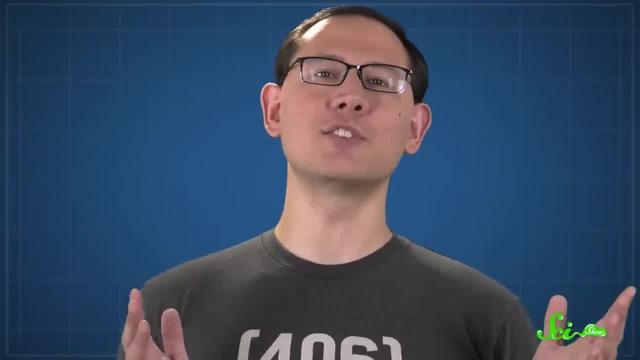 We can understand the behavior of the hundreds or even thousands of different types of particles that are created all the time in particle accelerators. And that's the kind of simplicity physicists strive for. Ah, physics. It's so beautiful, Just like a good spreadsheet or a really flexible Trello board.